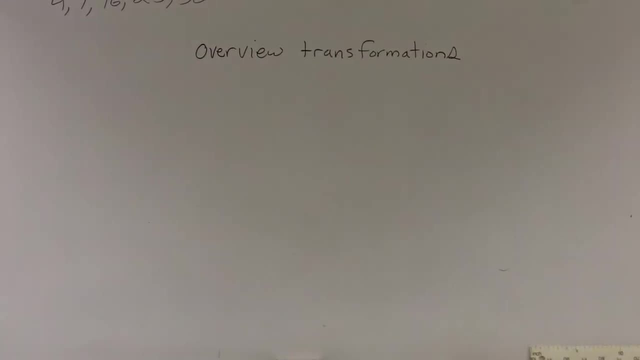 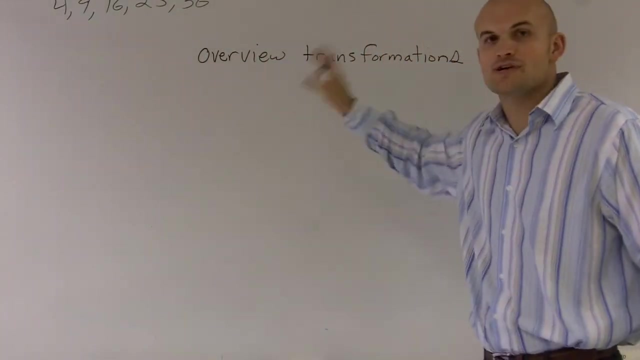 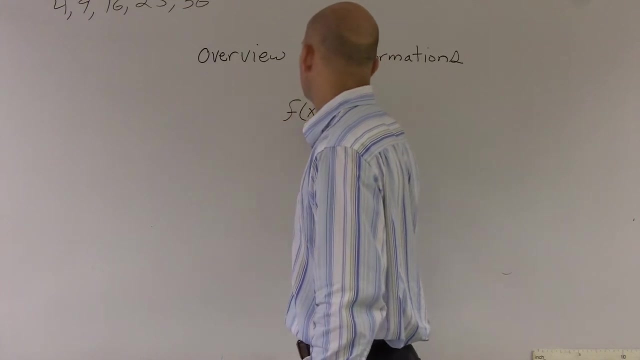 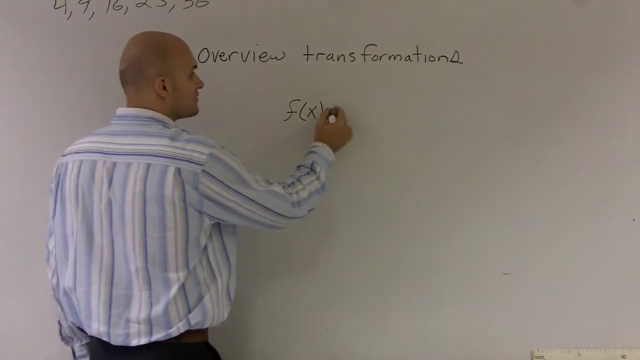 What I'd like to talk to you a little bit about is transformations. So first thing we've already previously talked about is functions, And there's many types of functions that we can have. We can have a constant function. we can have a linear function. f of x equals x. We've also talked 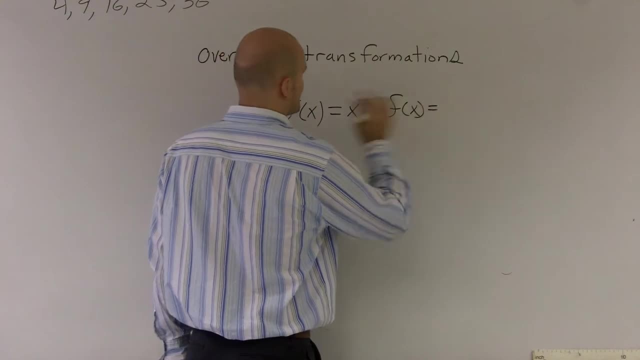 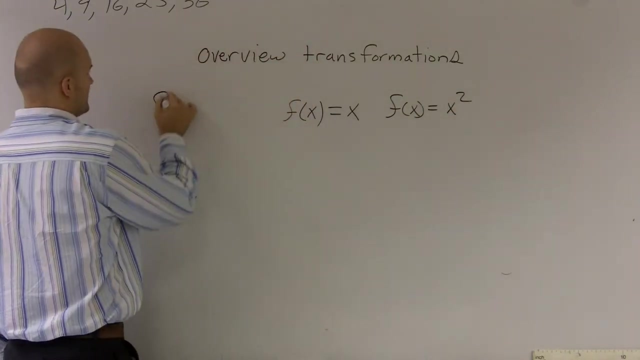 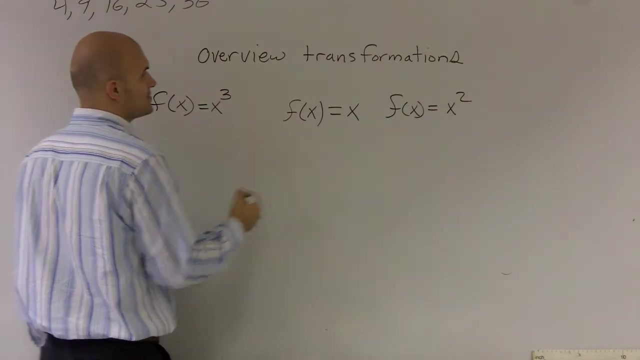 about quadratic f of x. I'm sorry. well, we'll just do it with a squared function, x squared. we have f of x. it's a cubic, And we can also do like an absolute value as well. We can also do a. 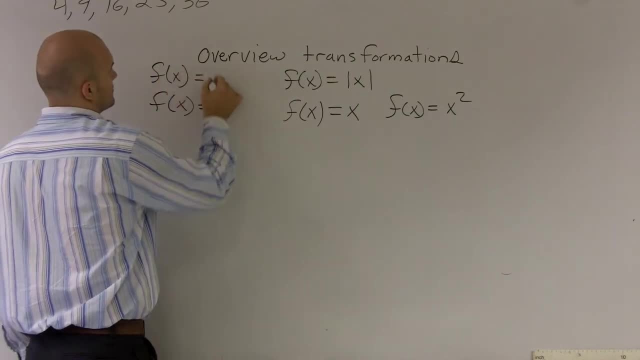 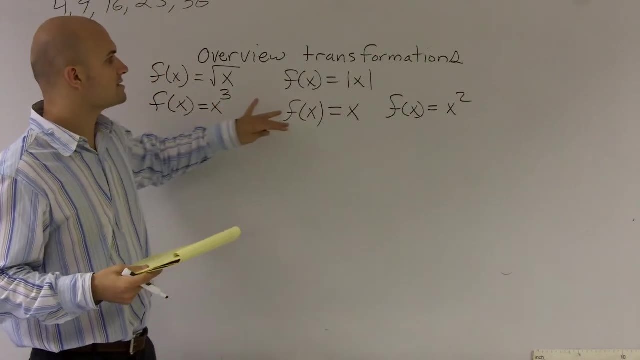 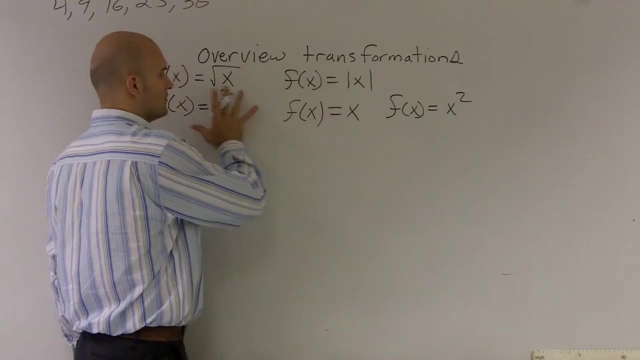 root. So there's multiple different functions And what, oh, oh, a lot of times what we've talked about in the previous chapter is: all these functions all have what we call a paragraph And they all have like a similar graph, you know, but without anything. 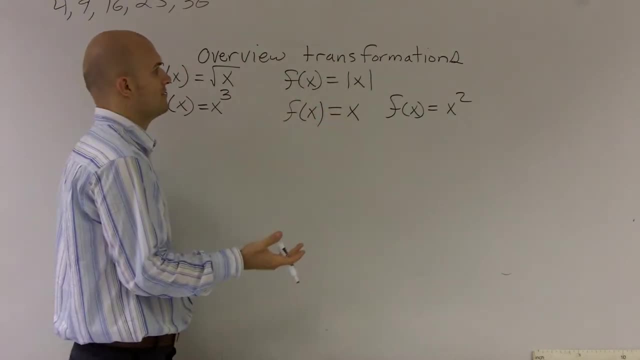 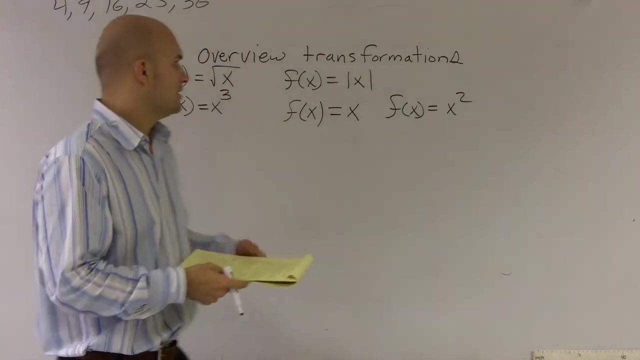 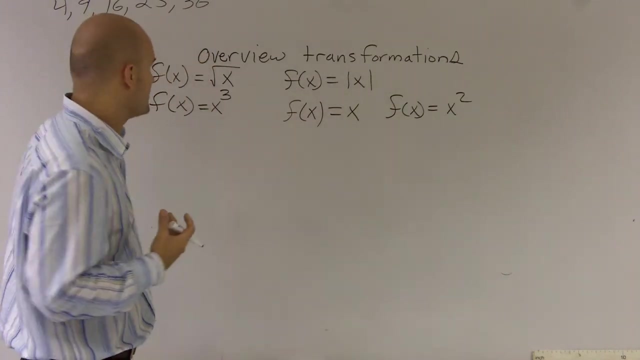 changing just what's happening to the x. we can draw a graph. Now what we're going to be working on is- or at least what we're going to give you an overview- is transformation, So pretty much saying: how are things going to change when we alter these functions? So for this problem, 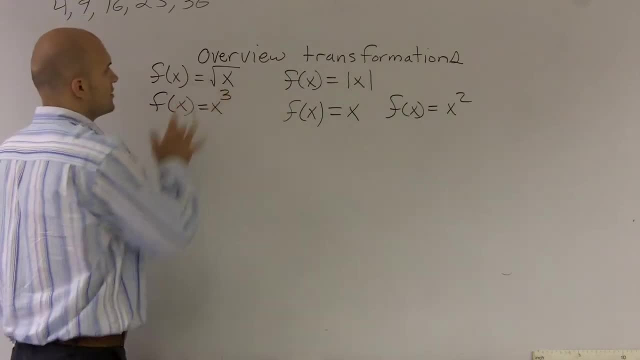 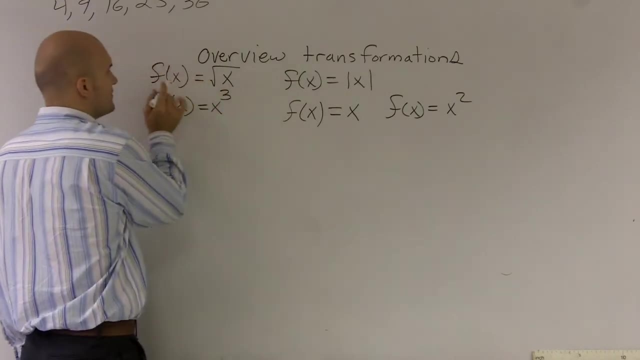 I am going to. I'm going to work with the square root function: square root of x. So the first thing we're going to talk about is I'm going to give, let's say, f of x equals square root of x. So I'm. 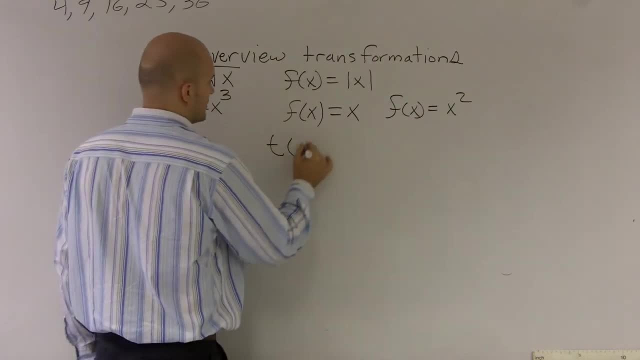 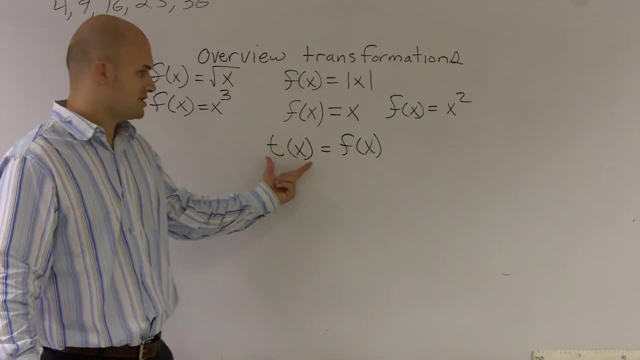 going to give a new function, which t stands for transformation of x equals f of x. Now, what we're going to do is so: this is my transformed function is going to equal my original function, which will be: let's see: 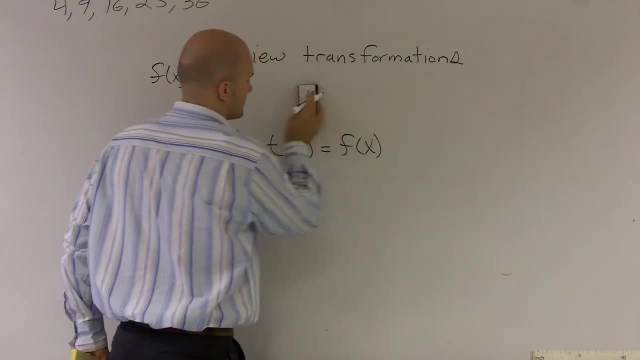 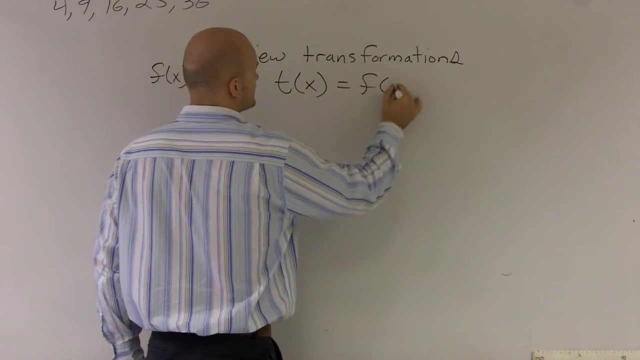 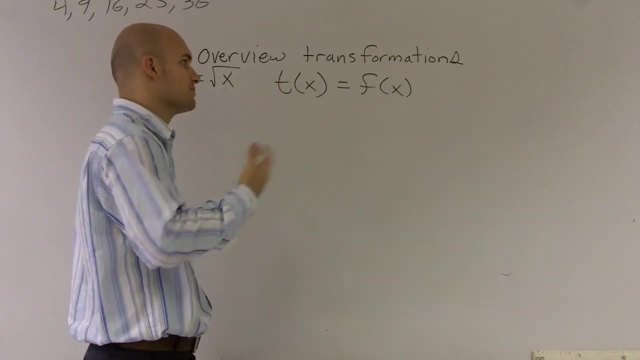 actually the rest of these, so we're not getting confused. Let's write: t of x equals my f of x, And what I'm going to do is I'm going to do a certain amount of transformations. So, and those, what those transformations we're going to call, we're going to, we're going to add with them c, So the 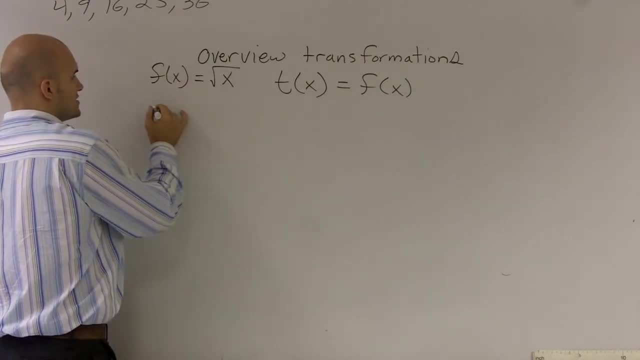 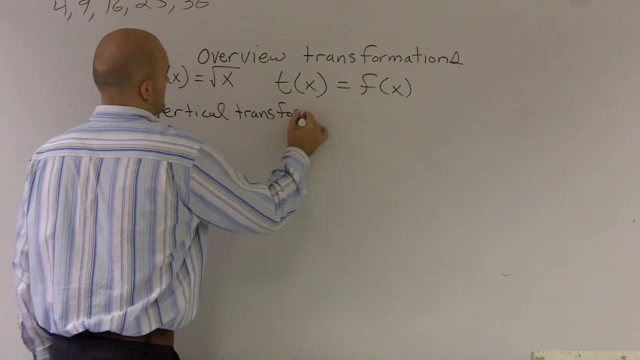 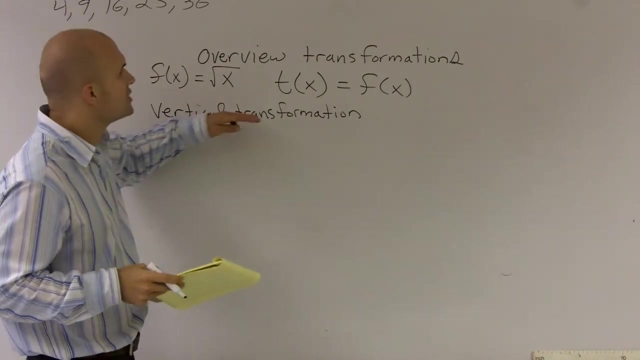 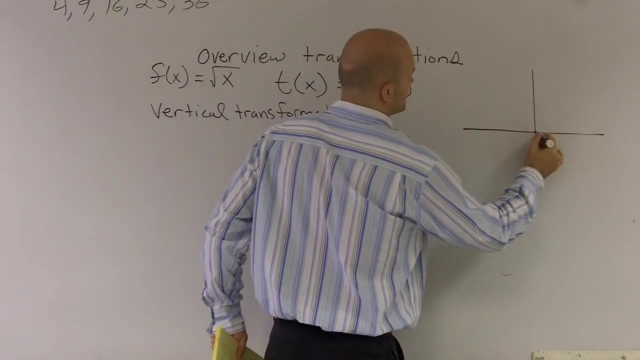 first thing, first transformation I'd like to speak about is vertical transformation, And a vertical transformations are pretty much when you're going to have a shift upward, downwards of the graph And a little bit of FYI. so if we have our original paragraph, the square root of 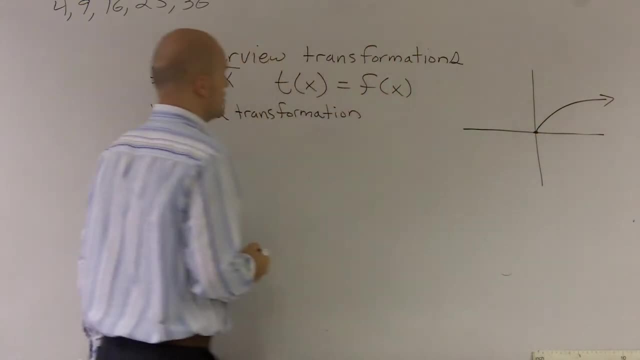 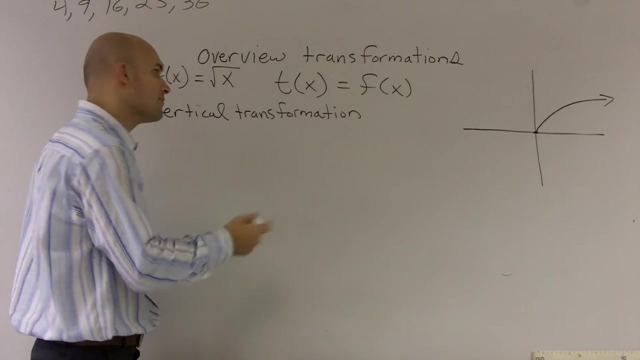 a function is going to look something like this: It starts at 0, 0.. So what we're going to do is: how are we going to represent, in a transformation of our original f of x, how can we represent a shift either upwards or downwards? Well, the way that we can do that is we're going to do a. 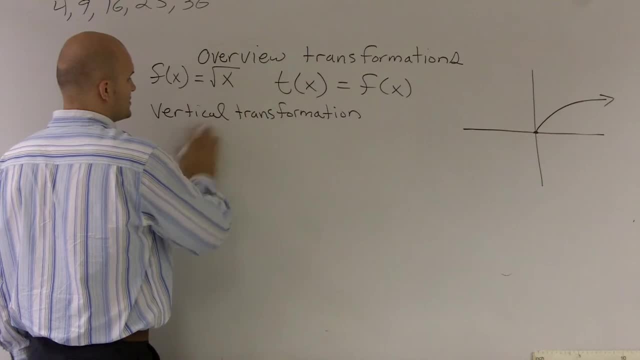 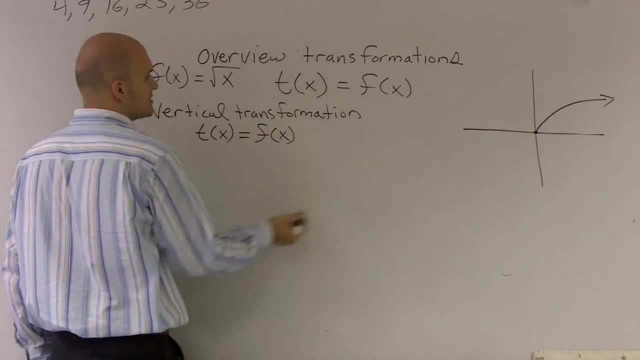 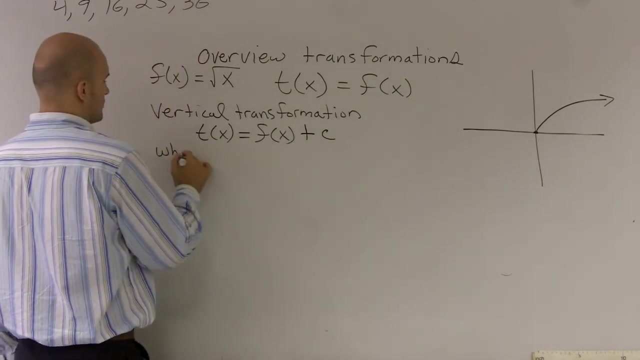 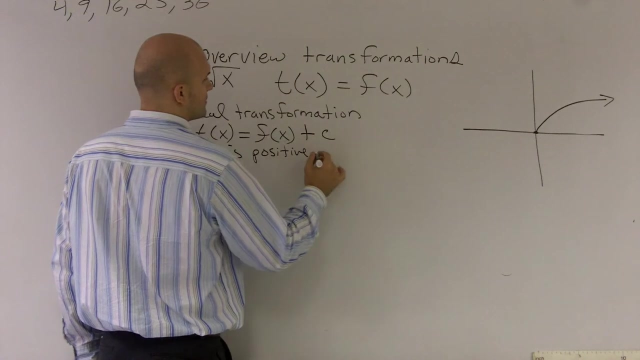 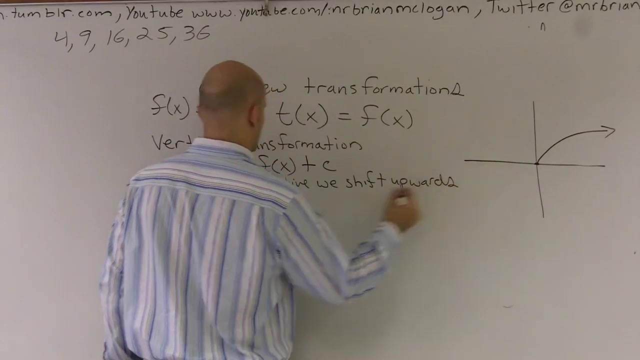 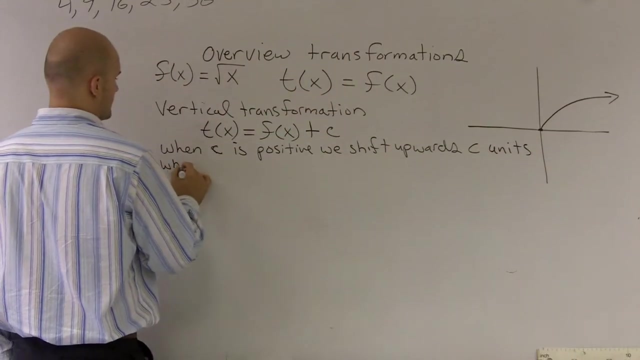 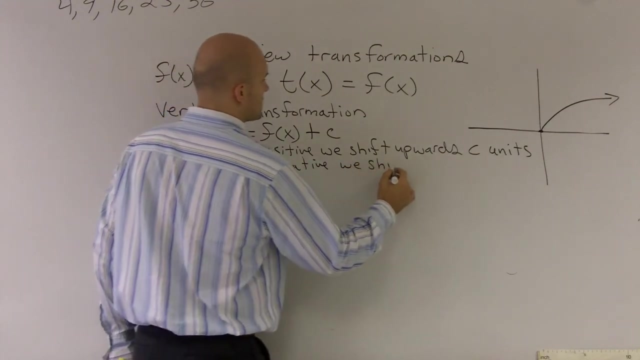 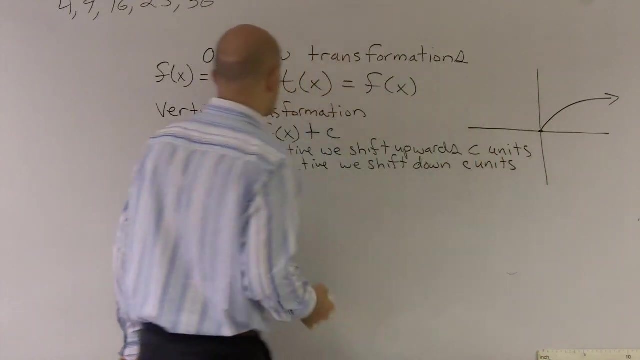 transformation of x equals my function f of x, and either we'll just say plus c, And when c is positive we shift upwards, So we shift down c units. And then we say when c is negative, we shift down c units. So for a couple, 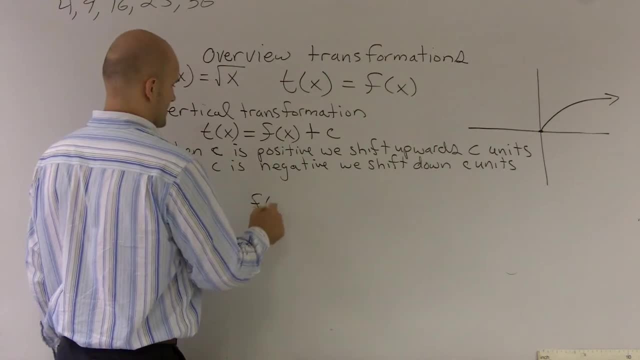 of examples. if I was going to say f of x is negative, I'm going to say f of x is negative. So if I was going to say f of x is negative, I'm going to say f of x is negative. So for a couple 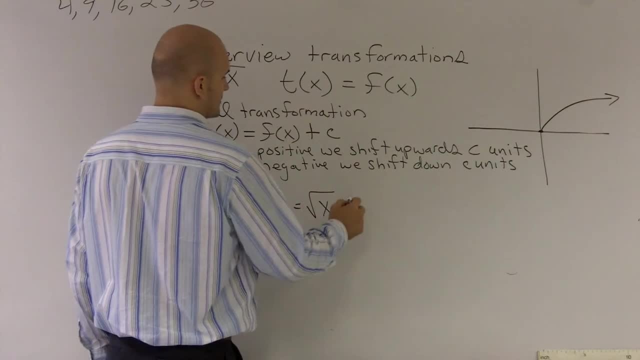 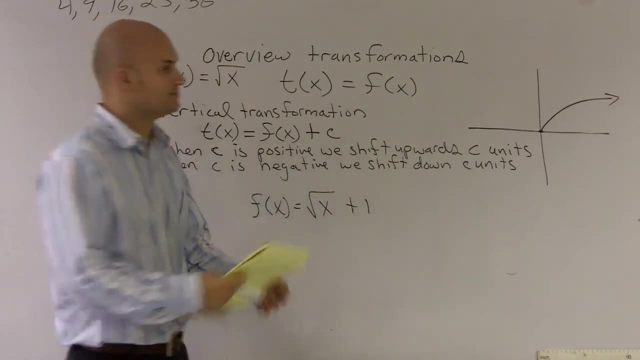 of examples. if I was going to say f of x is negative, I'm going to say f of x is equal to square root of x plus 1.. That would be shift my graph up one. So instead of starting at 0,, 0,, I would now start. 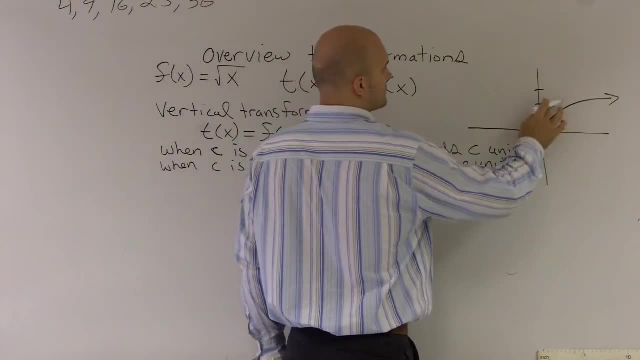 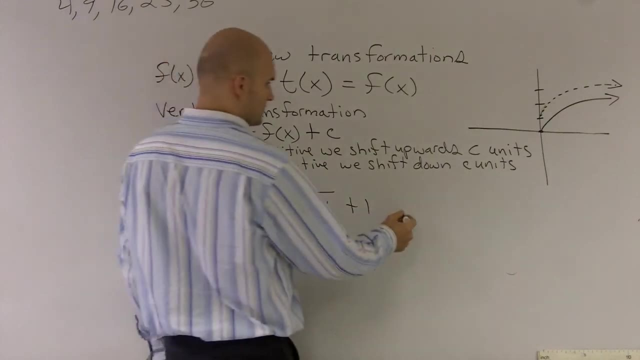 at 0,, 1.. And I would just graph- I'm going to just do a dotted line here And I'm just going to graph the exact same line. Let's do another example I could also do. let's do a negative 3.. 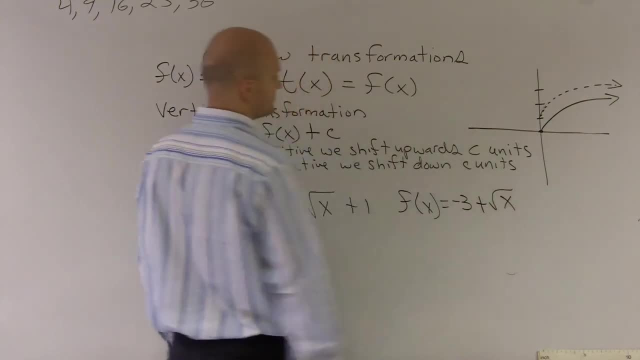 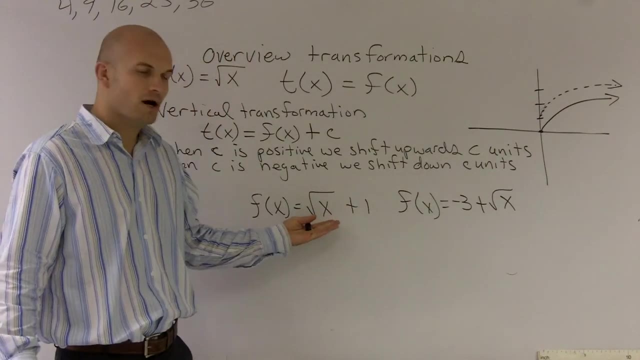 plus the square root of x. Now here I just tricked you a little bit and I just switched around the two forms, because usually we always write our variables always in front. But you know, in case sometimes you're doing some algebra or something.